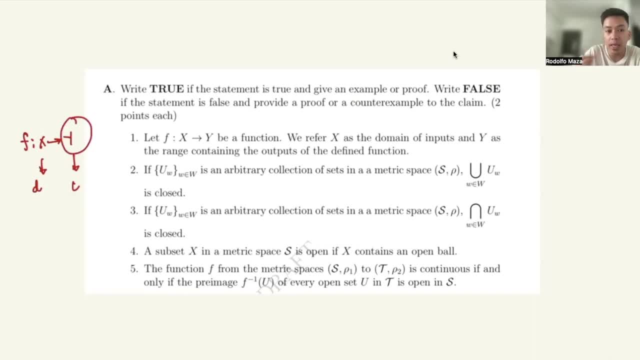 range, So hindi yung y mismo, kasi hindi naman natin sinasabi that the function is surjective, So therefore it's false. Number two: if this is an arbitrary collection of sets in a metric space, then the union of the collection is close Now. 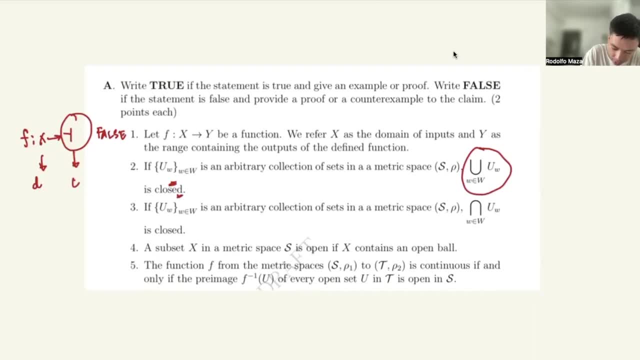 close kasi siya. So pag sinabi kasi natin ditong sets, ibig sabihin arbitrary sets, So how about those are open, So hindi siya magiging close. So therefore it should have to have close para mag-close din yung union niya Similar with. so this becomes false And 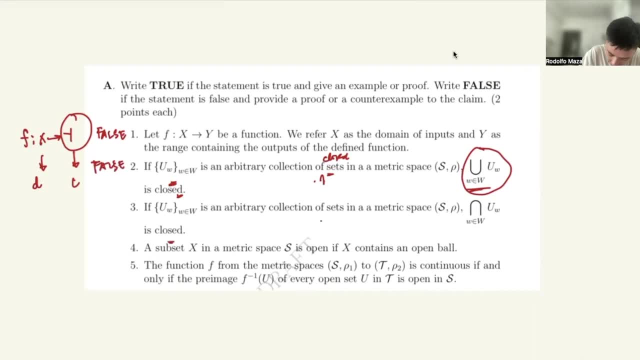 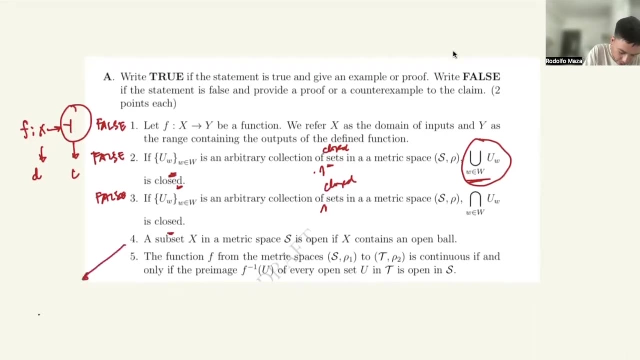 similar with number three. close kasi siya, So dapat i-close mo din yan, Kasi hindi naman pwedeng arbitrary sets lang. Okay, number four: a subset x. in a metric space, s is open if it contains an open ball, And we know this for a fact that if s contains an x, so yung. 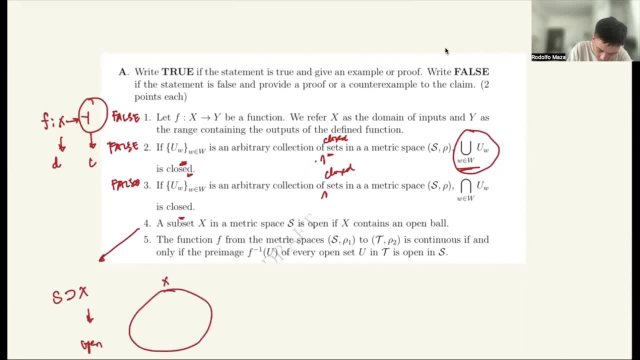 x mo magiging open Pag eto yung x mo, and then you have an open ball. let's say you have x there, So meron kang. let's say a radius of delta, So parang may open ball ka sa loob. We know. 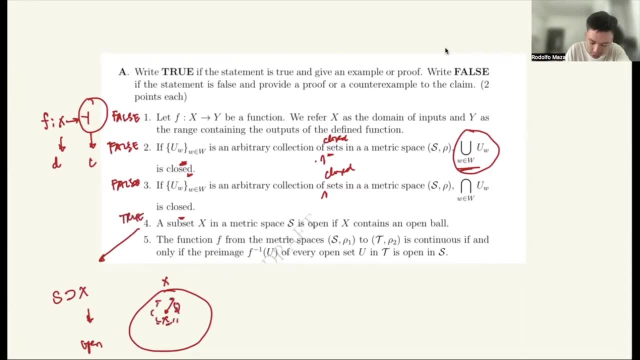 that for a fact. So therefore this is true. Number five, the function f from the metric space. this to this is continuous if, and only if, the pre-image of every open set u in t is open. And this is true. This is definition of continuity, So that one holds Okay, Okay. 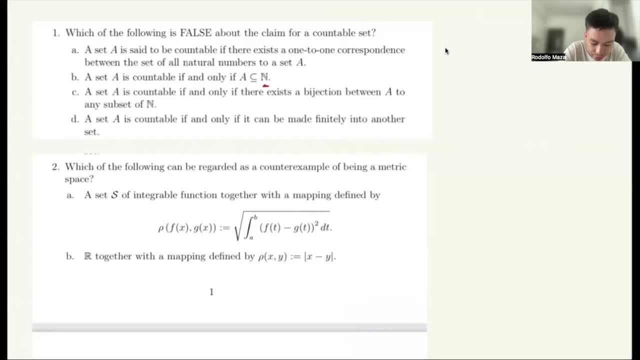 so for test two, which of the following is false about the claimant? So this is the definition of for a countable set. So kung titignan mo, number one, a set A is said to be countable if there exists a one-to-one correspondence between the set of. 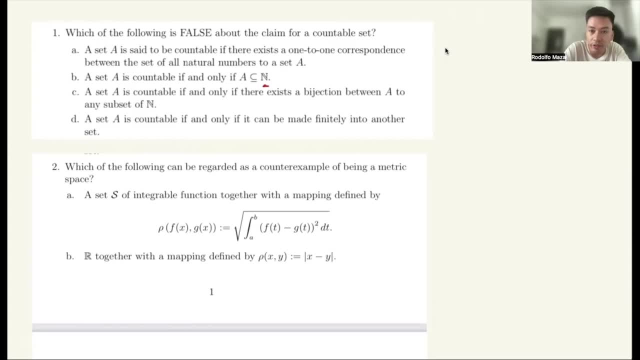 all natural numbers to a set, A. In fact, this is a definition for a countable set. So meron ka talagang one-to-one correspondence from your given countable set to the set of natural numbers. So this is actually true And A is countable if, and only if, A is a subset of. 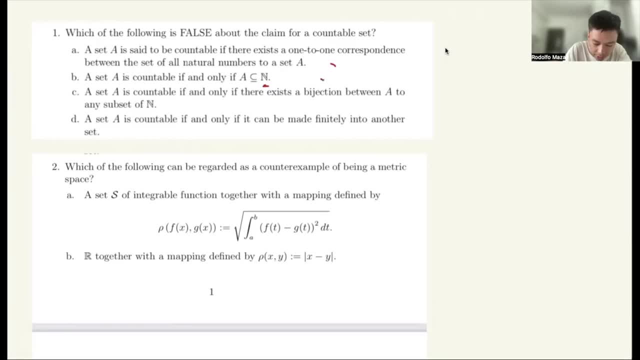 n. This is in fact true, And if A is countable, a set A is countable if, and only if, there exists a bijection between A to any subset of n, And this is actually a reinstatement, restatement of letter A. So 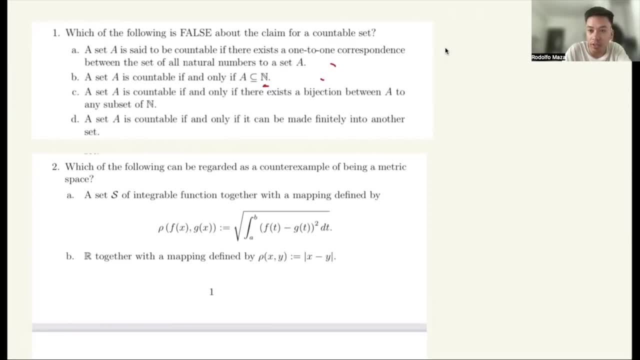 when we say it's a one-to-one correspondence, therefore it's a bijective function. So letter D, a set A, is countable if, and only if, it can be made finitely into another set. We can do that, We cannot do that. So therefore this is letter D. 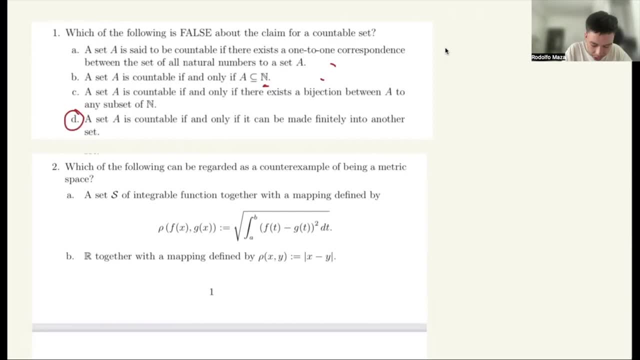 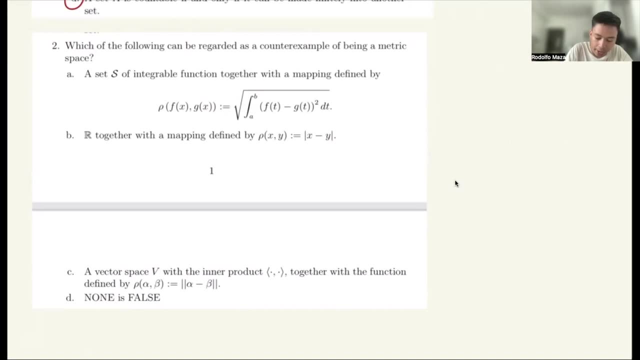 Okay For number two. which of the following can be regarded as a counterexample of being a metric space? So titignan natin sila. So paano nga ulit yun? Remember that for the rule for being a metric space, rho of xy is zero. So this is if, and only if, x equals y And 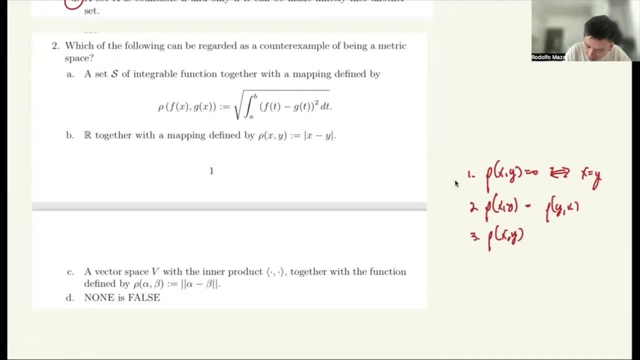 then number three, rho of xy. this should be less than or equal to rho of xz plus rho of zy. So this is triangle inequality diba. So we will check. Kung napapansin mo, if you equate f equals g, so yung rho niya magmaminus. 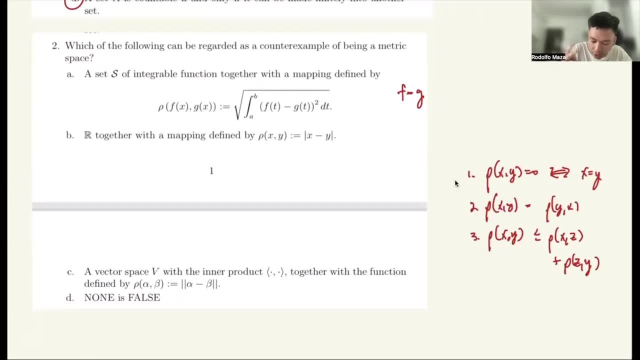 yan magiging zero, And that's actually true, And then pwede mo siyang iswap ang places nila, So magiging magswap siya dyan, Kasi square naman siya, so it's still the same, And then this is a function, so pwede. 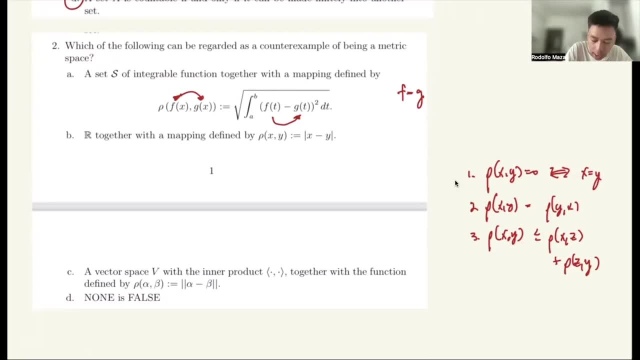 kang sisingit dun, and that's evidently greater than that. So therefore, this is a metric space For letter B naman, this one pag ganito diba: this is defined as the square of x minus y. Okay, Well, double check, Kasi. kung titignan mo, let us say ano ba at 3,, 1.. So 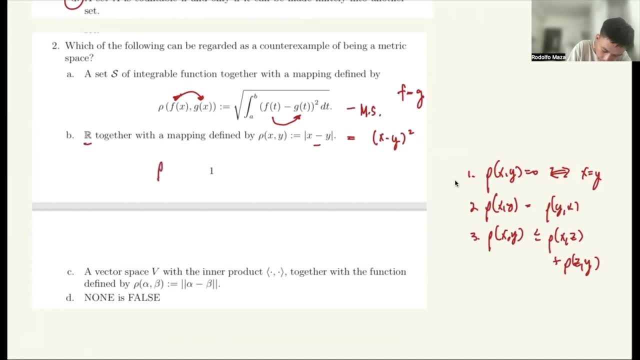 kunyari in R kasi. Okay, So that's rho of 3, 1.. So that's equal to 3 minus 1 squared, and that's equal to 4.. So, kunyari, sisingit tayo ng 2.. So rho of 3, 2,, and then plus rho of 2, 1.. So, diba. 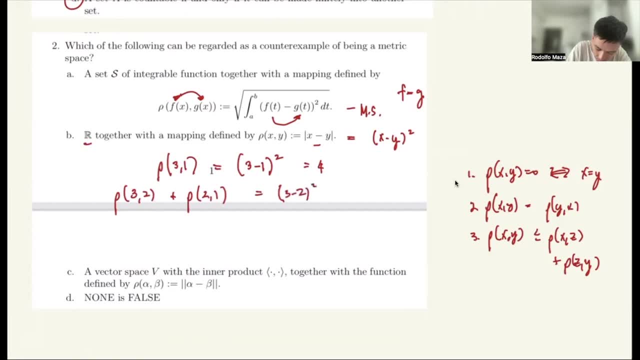 this is 3, 2? So ibig sabihin that's 3 minus 2 squared plus yung 2, 1, 2 minus 1 squared Diba, this is equal to 2 lang, and it's not greater than or equal to. 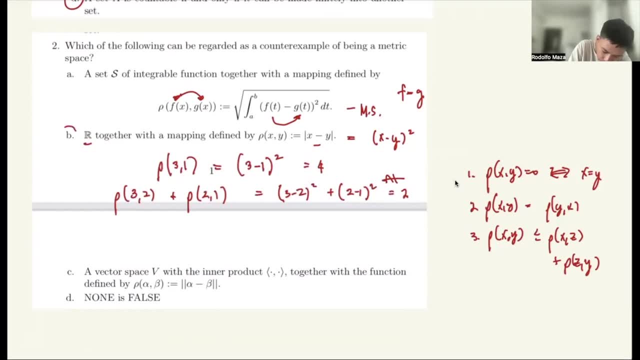 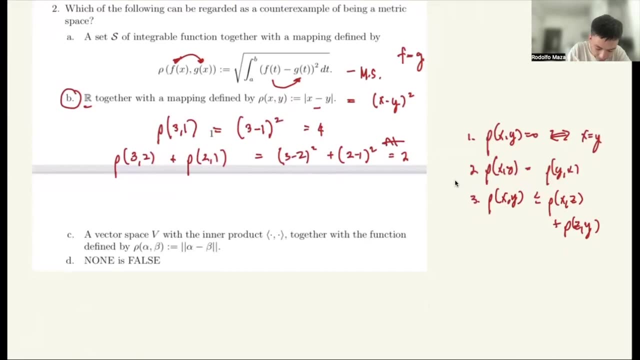 4. So therefore it disqualifies to be being a metric space. So number 3 kasi vector space. eh, So ibig sabihin, if your vector alpha is equal to the vector beta, then automatically the norm pala- sorry, of this- is zero, And then pwede mo siyang iswap kasi naka-norm. 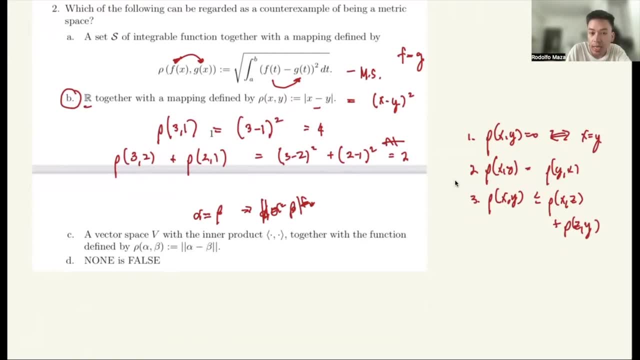 naman sila. and then the triangle inequality. pagsasali ka In fact isa to sa isang sikat ng isang example for being a metric space. So therefore the answer is P. Okay for number 3, which of the following is true for accumulation point? Point P is: 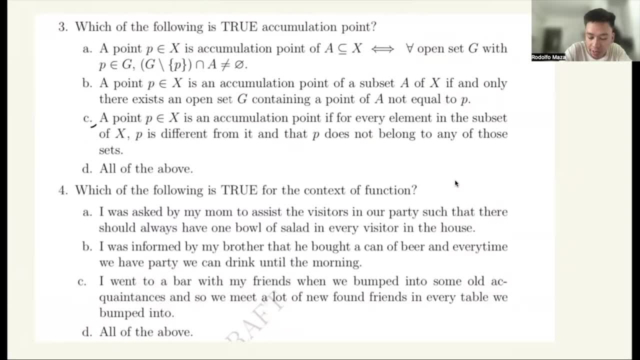 accumulation point of A, which is a subset of X, only for every open set G, This one holds. In fact, this is a definition of accumulation point. So mangyayari dito this is true? Eto naman, this is the same statement of letter A. so this is true, Kasi sabi dito it is. 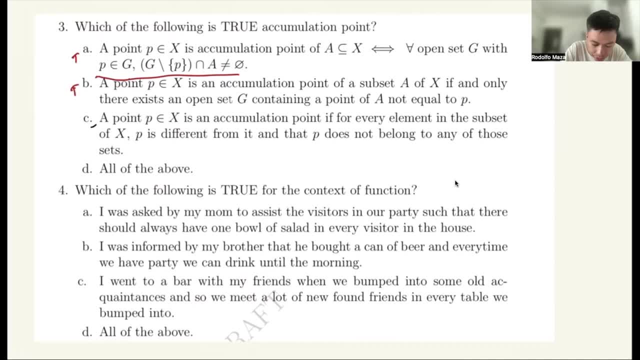 It is an accumulation point of a subset A of X if, and only if, there exists an open set. So this open set, G in A, it's the same, but it contains a point of A not equal to P, It's the same as having. the intersection is not empty. so therefore it's true. 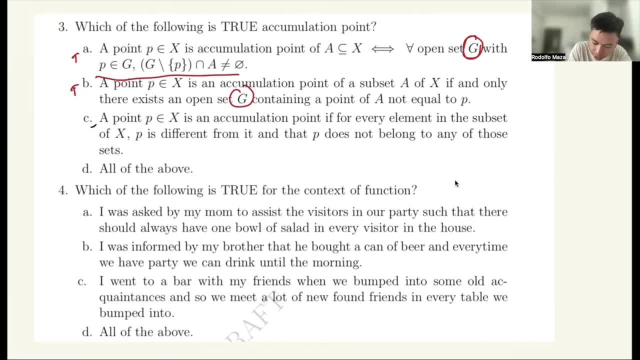 For letter C, a point P in X is an accumulation point. if for every element in a subset X, P is different from it and that P does not belong to any of those sets, It's not necessary that it's not in the sets. it can be there. it can't be not there. 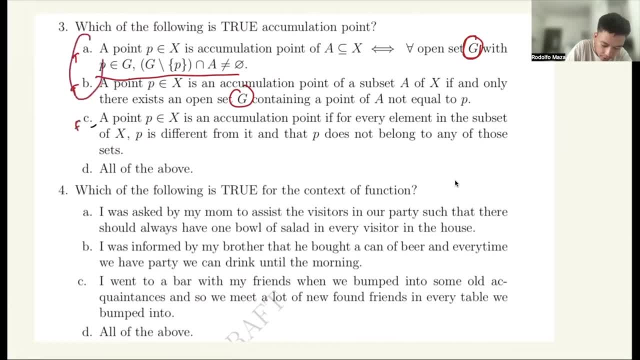 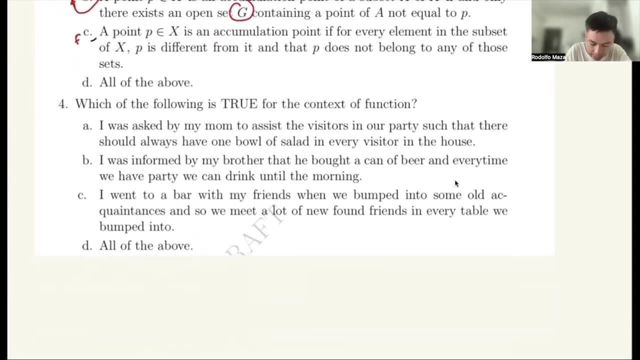 So, therefore, this is false. So the only true here is this. Number four, which of the following is true for the context of function: I was all asked by my mom to assist the visitors in our party such that there should always have one bowl of salad in every visitor in the house. 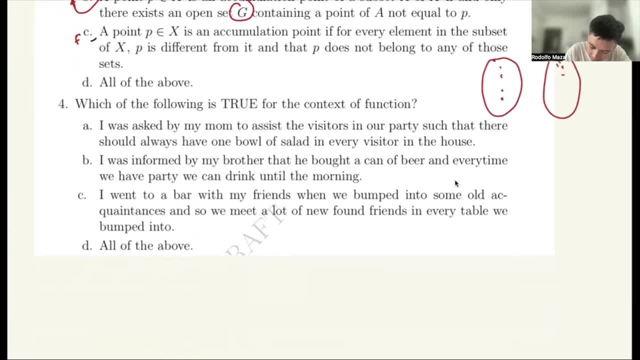 So you have a visitor here and you have a. So it's like it says: there is a correspondence for every visitor to have a salad. So therefore it's a function. Letter B: I was informed by my brother that he bought a can of beer. 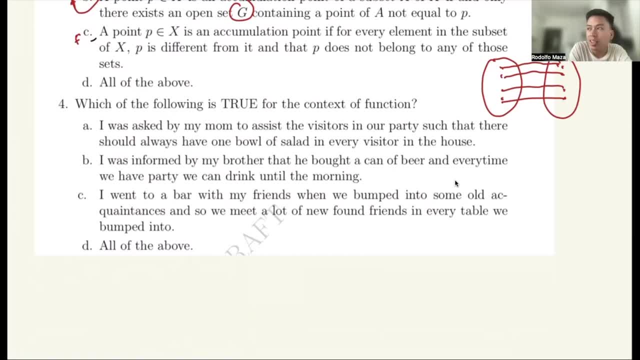 and every time we have a party we can drink until the morning. There is no message on this, like it's very ambiguous, So it means that it's not really declared as a function. Number three: I went to a bar with my friends when we bumped into someone. 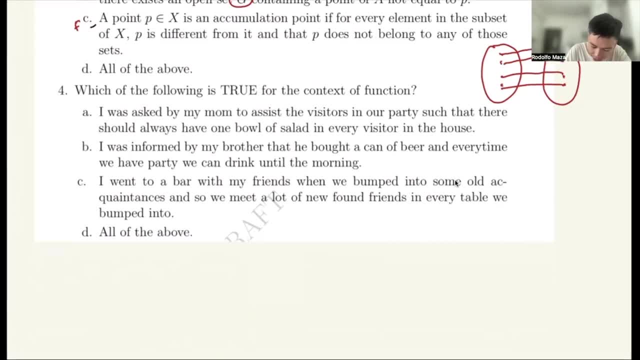 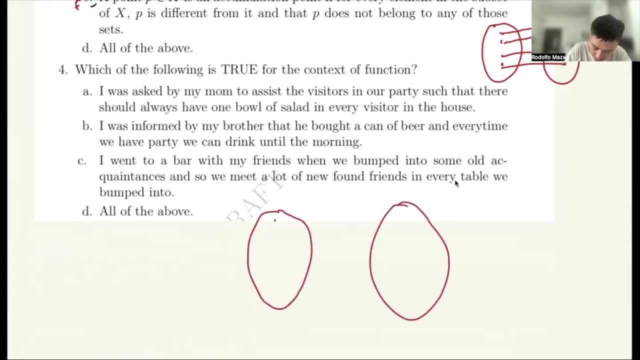 called acquaintances, and so we meet a lot of newfound friends in every table We bump into. it's still ambiguous, because if it's you, then these are the bars, So it means Okay. so number five: which of the following is not a topology, on X having three distinct elements? 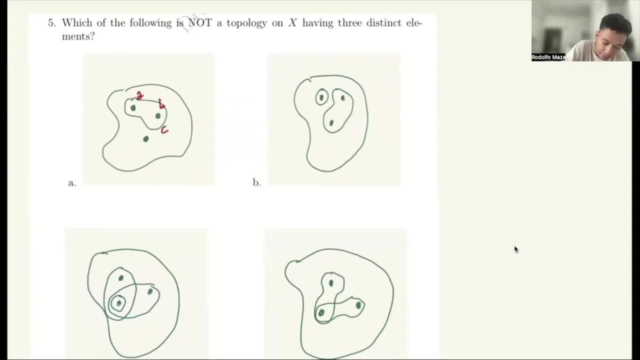 So if this is your A, this is your B, this is your C. So it means that the person here contains the M, T, the X, your A, B and the C. Oh no, this doesn't have a C. 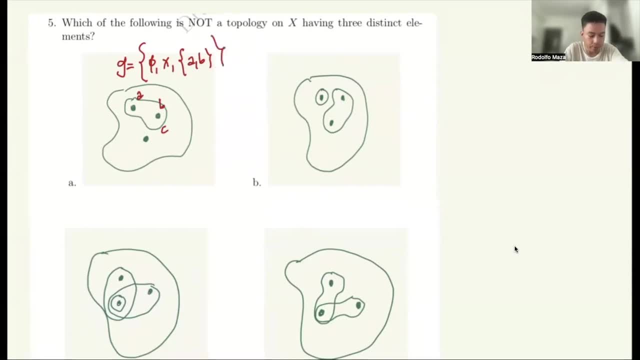 So that's it. So, if you're going to prove it, that is a topology, because we know that the intersection is there, empty. The union is there, the intersection with this, this one, and then the union is the X itself. 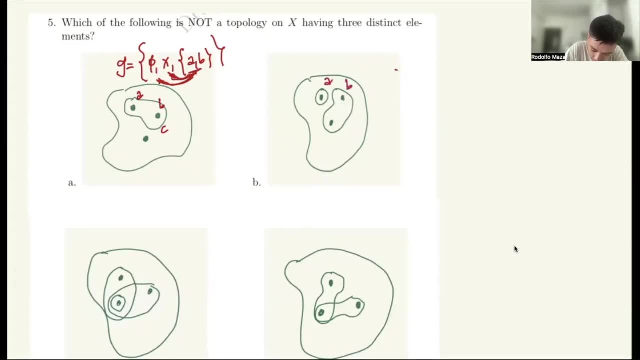 And for this letter B. so for example, this is the A, B and C. So your tau here is the M, T, the X, the A And the B, C. So if you take the union here it will be X. 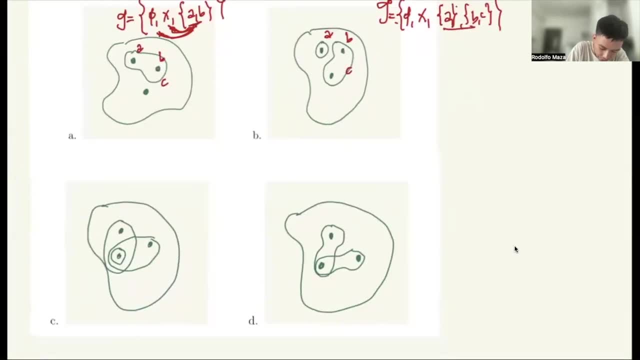 If you take the intersection it will be empty, So that's correct. For letter C, for example, this is A, B and C, So your tau is the M, T, the X, the A, C, the B, C and the C itself. 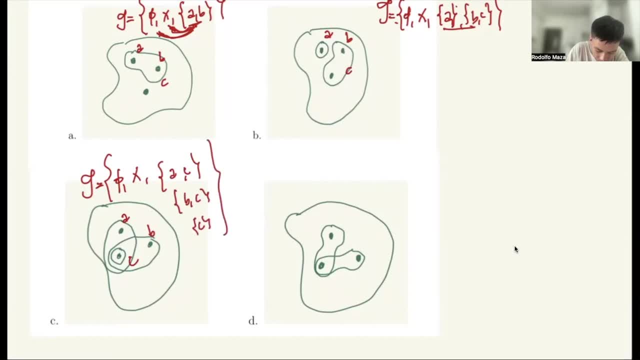 So if you take the union of these three- A, B, C- If you take the union of these two- A, B, C, still, If you take the intersection of these, C is here. So therefore it's a topology. 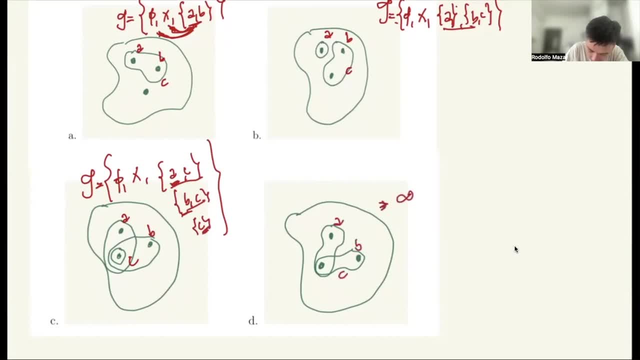 This is A, B C, So your tau is M, T, the X, What else? We have A C, We have B C, But if you take the intersection it should be C. It's not there. 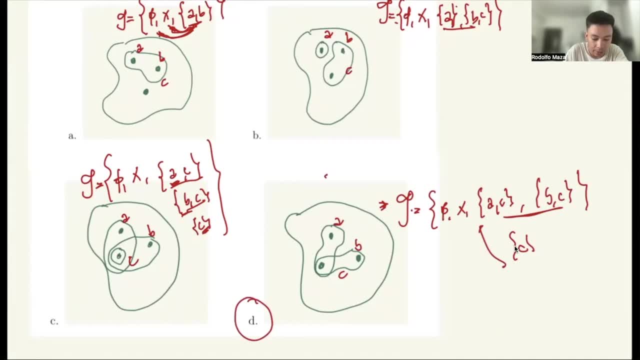 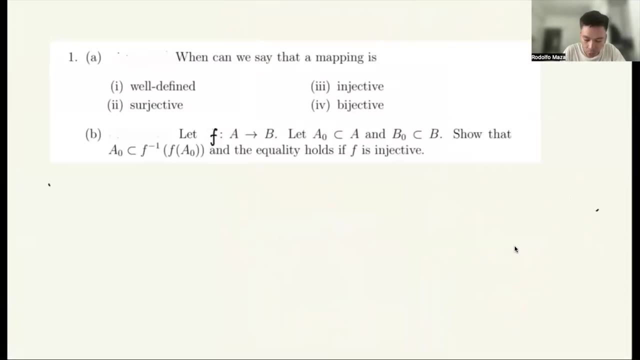 So therefore, this is not topology. So the answer is letter D, Because we're looking for, not a topology. Okay, so let's go for test three. So for test three, when can we say that a mapping is well-defined? So parang pinasasabi tayong definition, no, 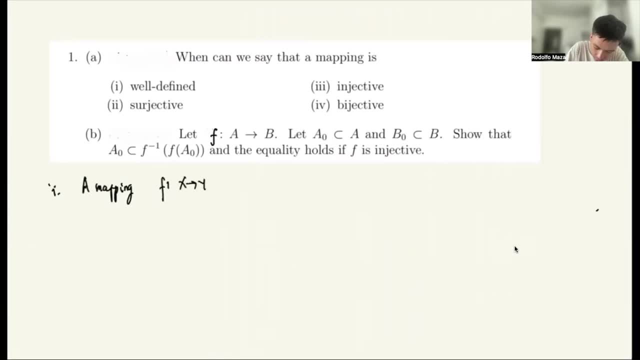 A mapping F from X to Y is well-defined. Yan Paano naging well-defined If, for every X in X, there exists a Y in Y, Such that F, If F of X equals Y and if X sub 1 is equal to X sub 2,? 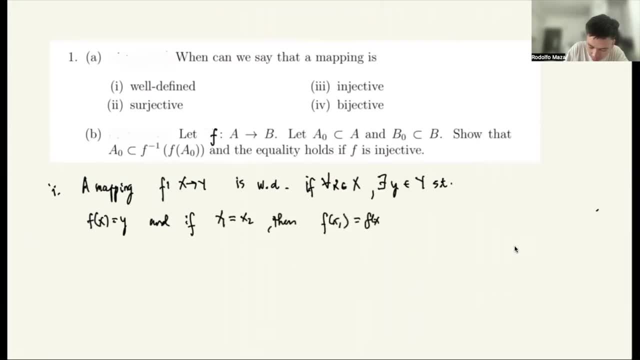 then F of X sub 1 is equal to F of X sub 2 for all X1 and X2 in X. For number two naman, F a function. F is surjective Yan, So diba pag surjective mag i-equal yung range at yung domain. 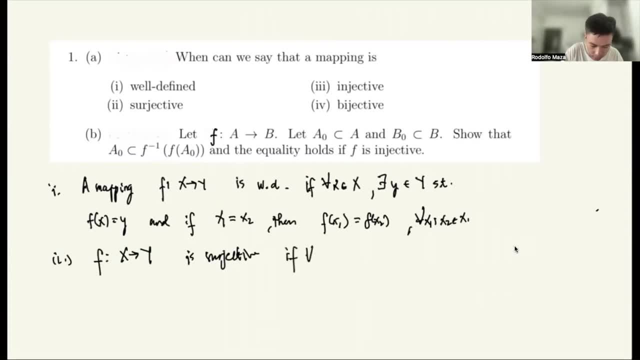 So this becomes surjective If for every Y in Y, so ibig sabihin lahat ng elements sa Y, there exists X in X, such that F of X equals Y, So lahat ng elements ni Y na mamap kay X. 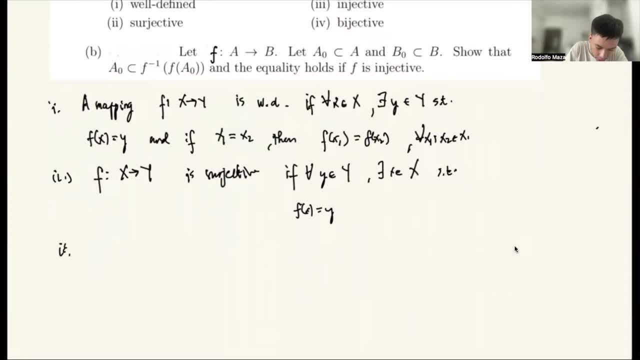 So that makes it surjective. So number three is: F is injective. If F of X is equal to F of Y implies X equals Y Diba. eto naman, yung talaga nagpuprove tayo dati. 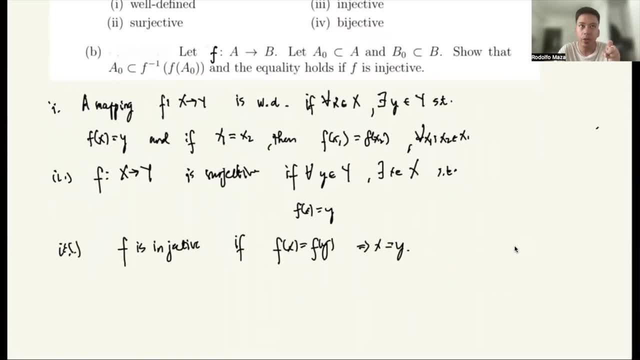 Like you're given with a locus and then you're asked to verify if that function is actually a one-to-one or injective. So ibig sabihin diba i-equate mo siya sa F of X equals F of Y. 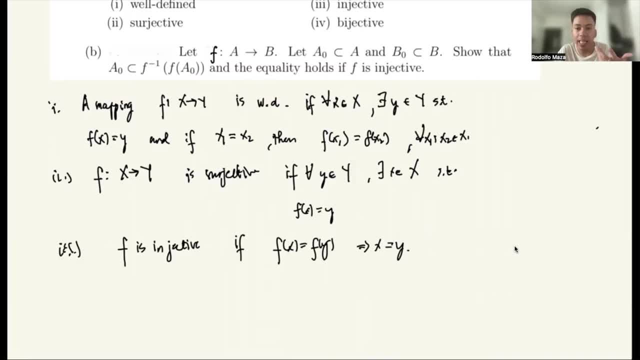 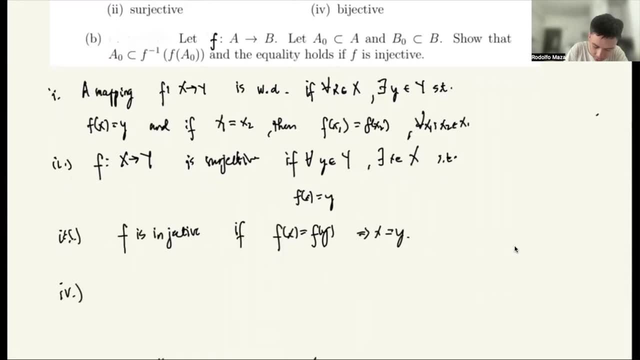 and then your conclusion should have: X equals Y. So yun naman talaga yung pagpuprove. And then number four, So magiging bijective siya if it's both surjective and injective. So we know that for a fact that a bijective function is an on-to function and a one-to-one function. 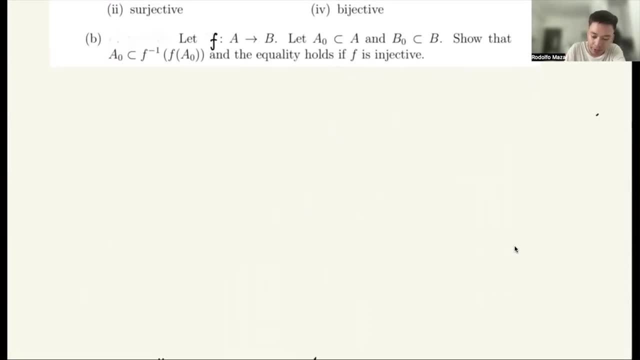 That's it. How about for letter B? So yung letter B let F from A to B and then A sub zero is a subset of A and B sub zero is a subset of B. Show that A sub zero is a subset of F, inverse of F of A sub zero. 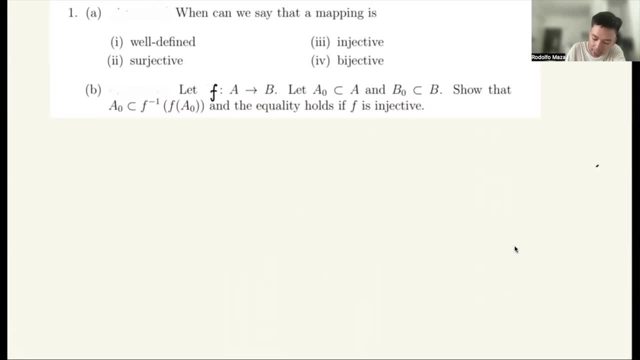 and that equality holds if F is injective. So paano yan? Probe natin, I'm drop lang to ha. So let X in A sub zero, So anong magiging mangyari yan? So then yung F of X mo is an element of F of A sub zero. 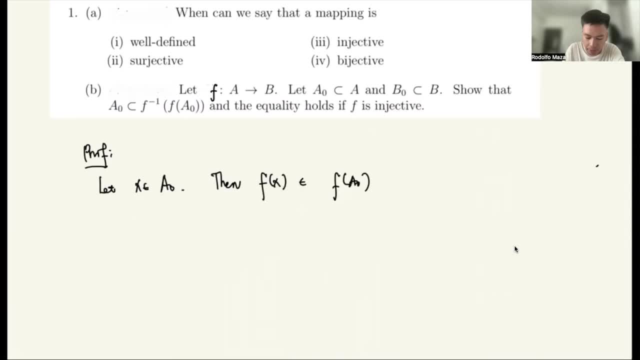 Tama, Okay, By definition of a function. And then anong mangyari? Itadrop ko na lang to So mag-a-araw lang ako F inverse of F of X. So that's the same as element of F inverse of F of A sub zero. 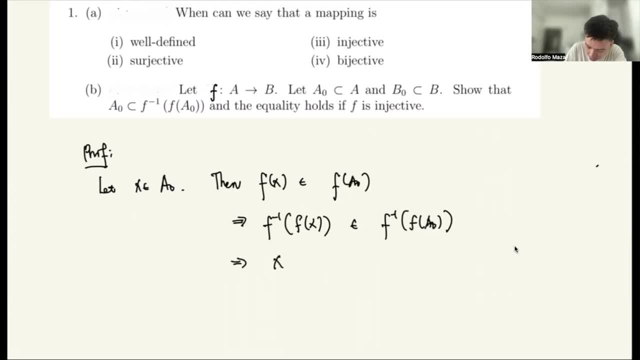 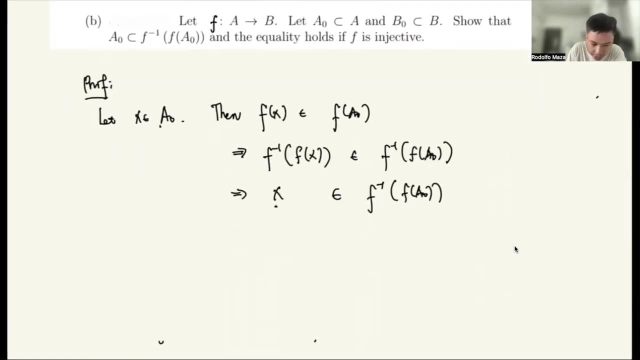 What is F inverse of F of X? Di ba that's X. So ibig sabihin it's an element of inverse of F of A sub zero. So dahil yung X mo nagaling kay A sub zero, naging element niya dito. 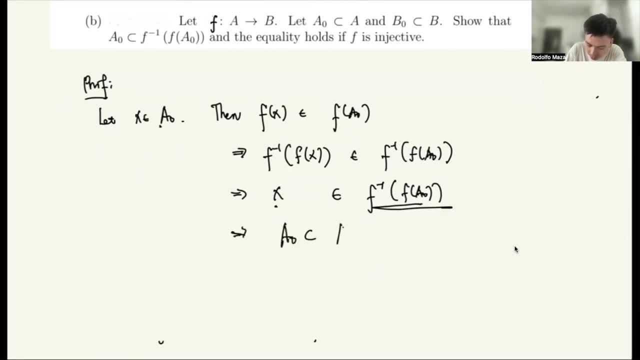 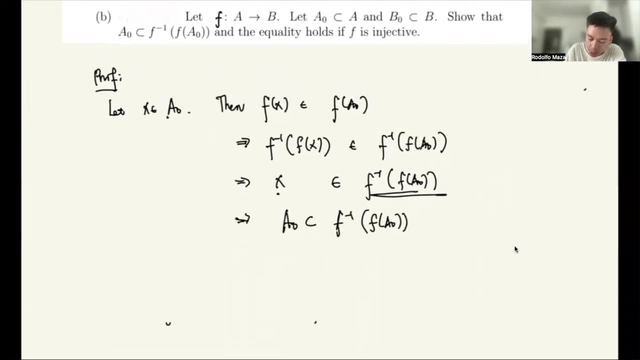 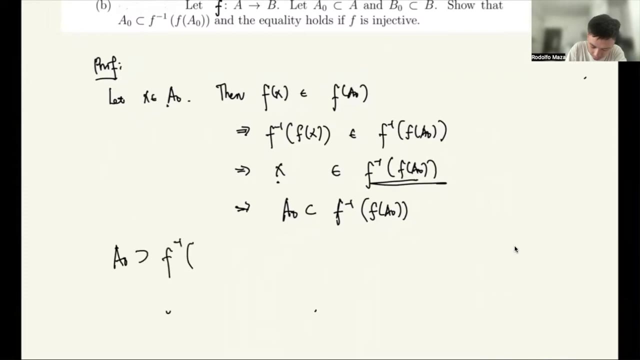 So the conclusion is: A sub zero is a subset of F, inverse of F of A sub zero. Okay, Now the equality holds if F is injective. So ipapakita mo na yung A sub zero also contains F, inverse of F of A sub zero. 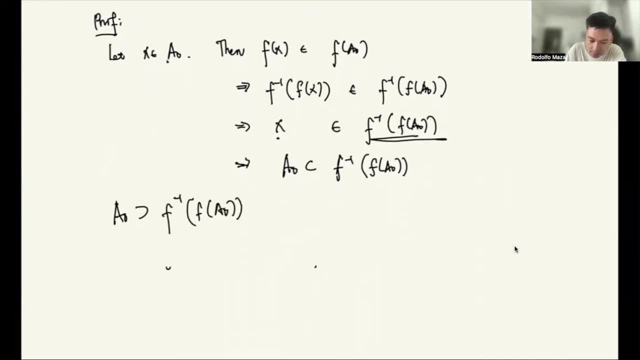 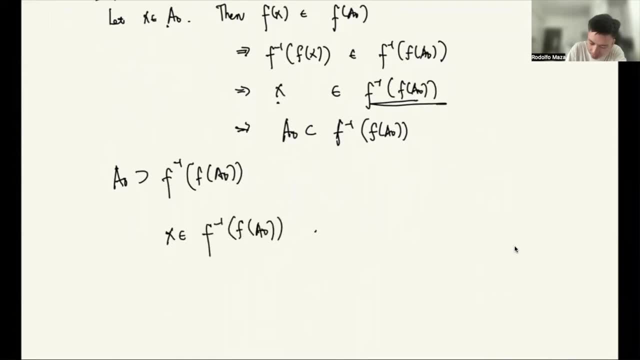 And this holds only if F is injective. So paano yan Sige nga Let X be element of F, inverse of F of A sub zero. Di ba Dito tayo magkukuha Tapos yung conclusion natin, dapat makikita natin yung X dyan. 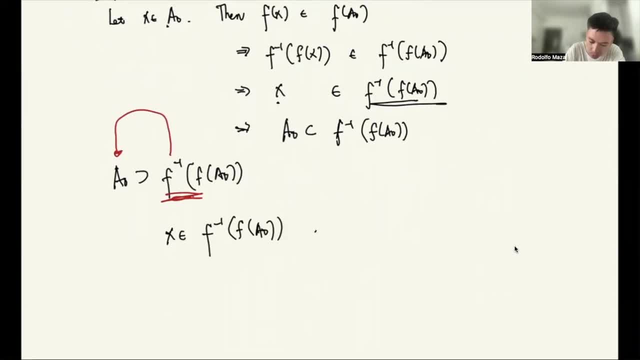 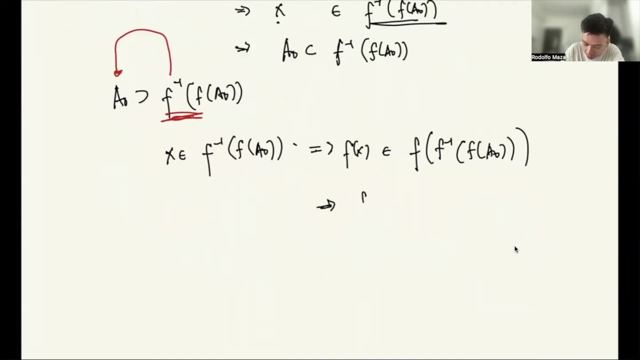 Okay, Paano. So implication nito: this is F of X, element ni F of F, inverse of F of A sub zero, Tama. And so this implies F of X is an element of, so mawawala to this is F of A sub zero. 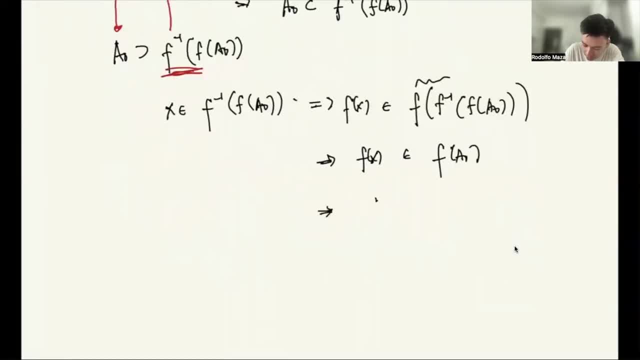 Tama, no. So ibig sabihin, yan F of X is equal to F of Y. sige, gamit tayo ng ibang variable X sub zero, na lang For some X sub zero in A sub zero. 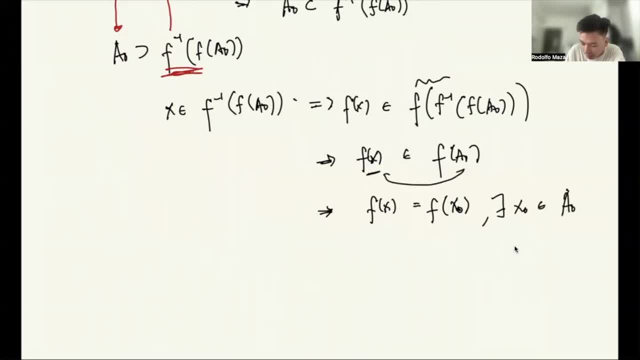 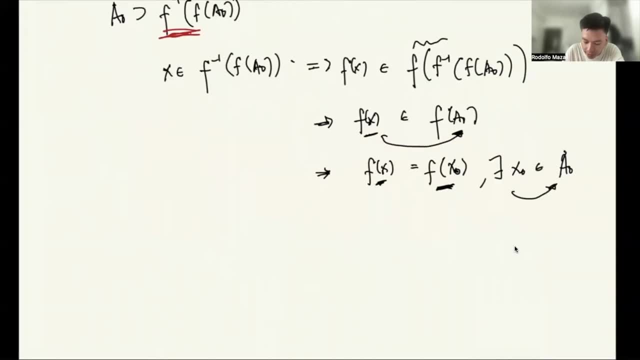 Tama Kasi di ba dahil ito element niya, ibig sabihin, ito can be equal to some like this na nang dun dyan, Pero since F is injective, since F is injective. 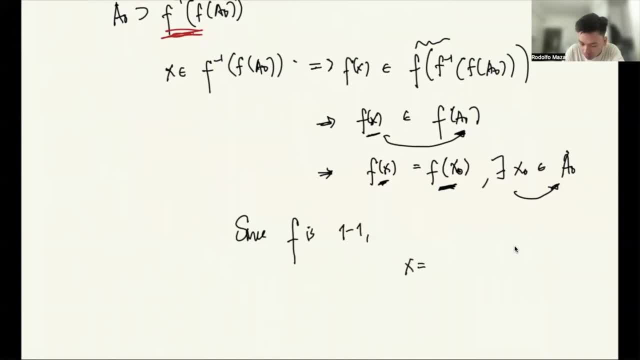 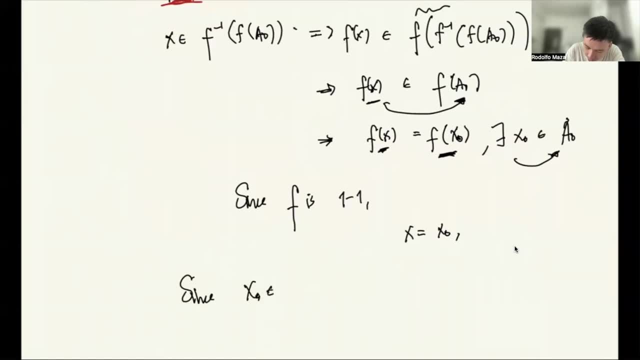 ibig sabihin X is equal to X sub zero. So since X sub zero is andun kay A sub zero, it follows that X is an element of A sub zero. So this implies yung F- inverse of F- of A sub zero. 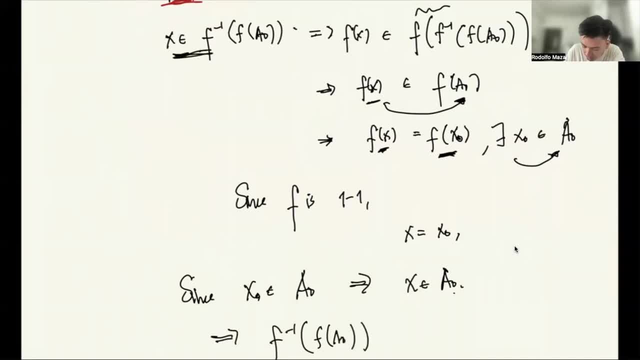 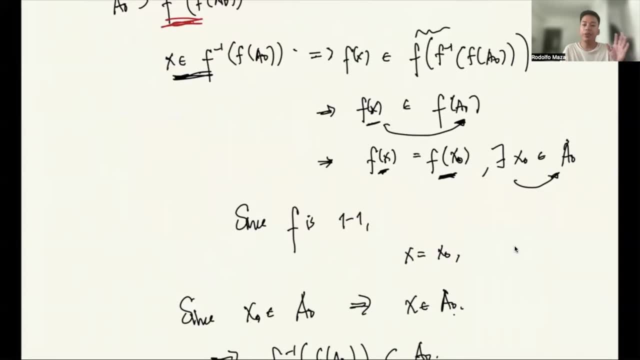 kasi di ba element niya yung X, pero naging element ni A sub zero. So it's a subset of A sub zero. So therefore equal sila. Okay, So if you have any questions or clarification. 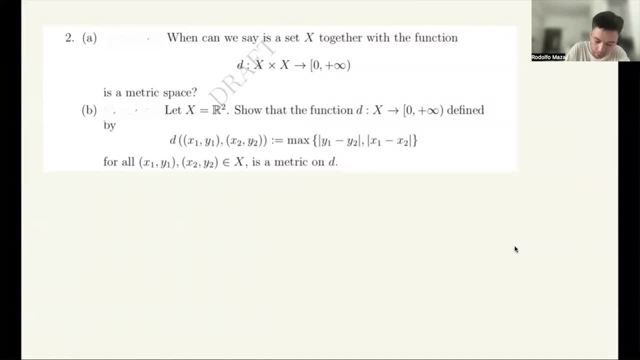 please let me know. So how about, for now, Number two. Okay, for number two. when can we say that X together with a function? this one is a metric space. How do we define that A set X together with the function? 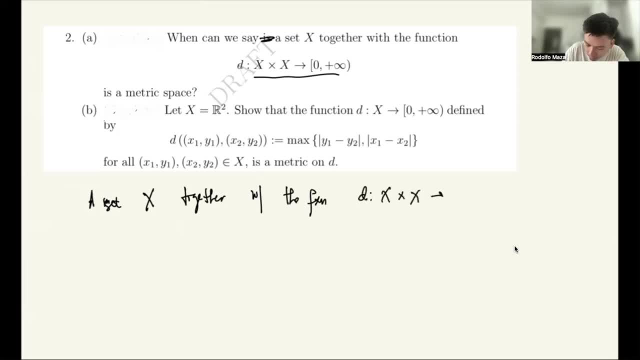 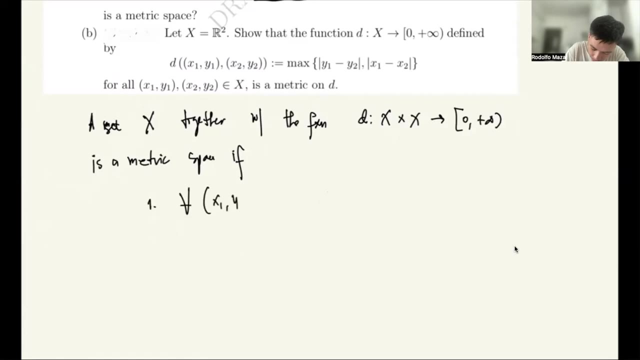 D, X cross X to zero. infinity is a metric space. If the following are satisfied, completely satisfied, number one for every, for every: X1, Y1, and X2, Y2 in X cross X with D of X sub 1, Y1, X sub 2, Y2. 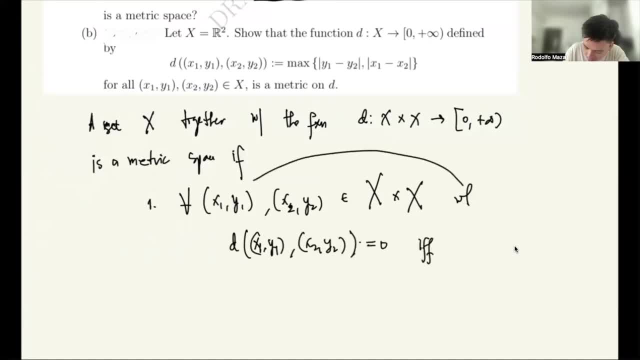 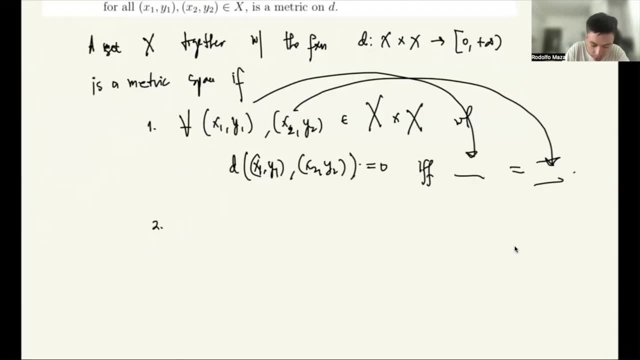 is zero. if, and only if, eto siya, surat ko na lang dyan, eto siya, they are equal. Okay, number two, yung D of X1, Y1 mo, X2, Y2 mo. 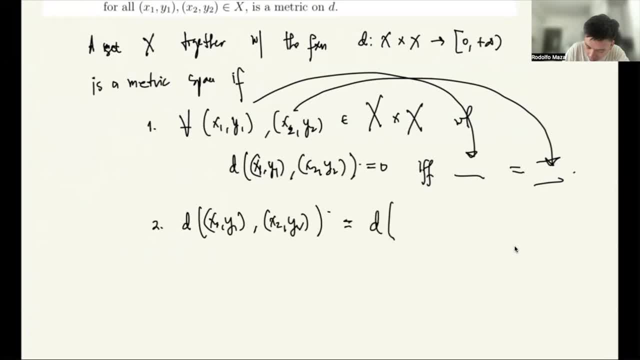 is the same as D of X2, Y2, X1, Y1.. And number three ano ngayon: D of X1, Y1, and X2, Y2,. this is less than or equal to D of X1, Y1,, X3, Y2, Y1. 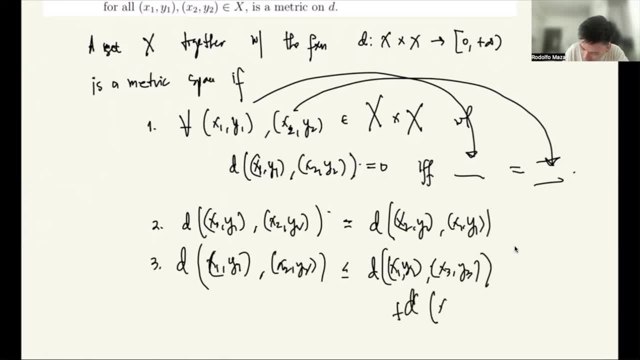 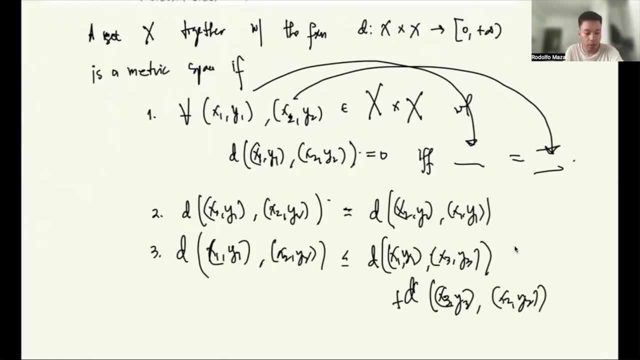 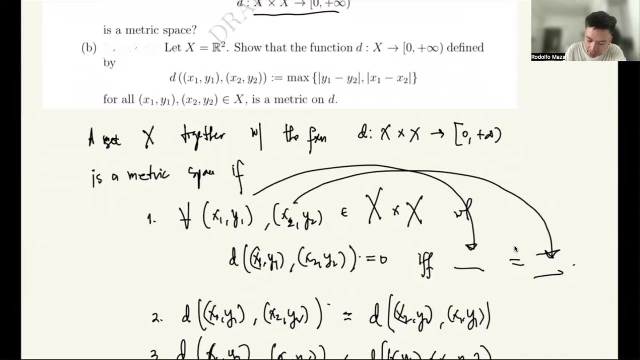 Okay, y3 plus D of X3, Y3, X2, Y2.. Okay, So that's the definition, lang. Okay, For now. letter B show that the function defined by this is a metric space. So, madali lang, to. 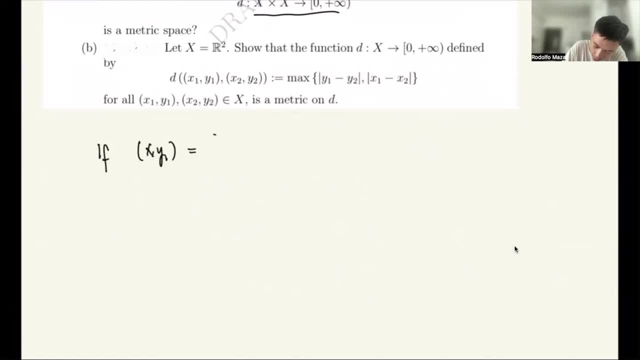 Paano ba, If X1, Y1 is equal to X2, Y2, then X1 is equal to X2, so Y1 is equal to Y2.. Thus ano mangyayari D of X1, Y1,. 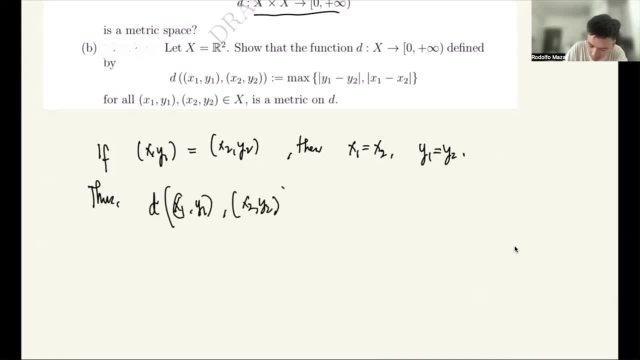 D of X2, Y2,. this is the same as the max of Y1 minus Y2, and X1 minus X2.. Yan So Y1 minus Y2, because they are equal, so that's equal to zero. 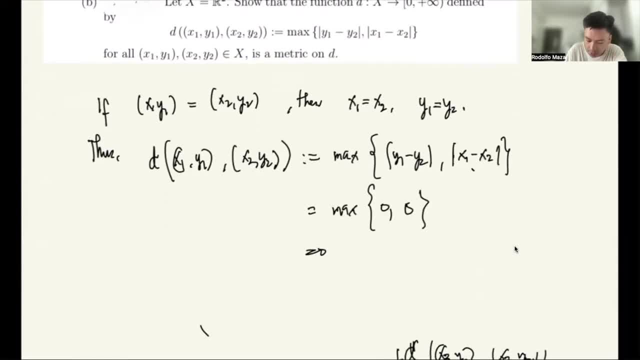 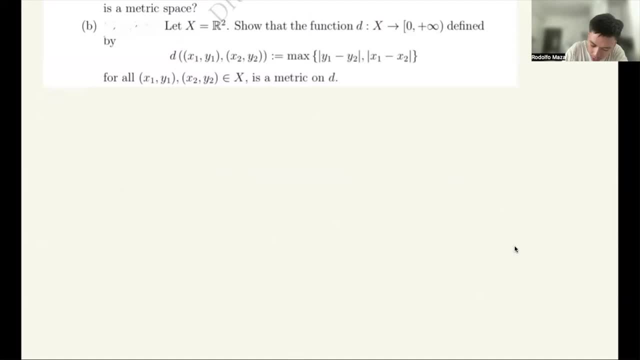 Ito naman zero, So the max is zero. Okay, So condition 1 for a metric space is satisfied. How about condition 2?? So let's try. Actually we can swap Dito ko na lang titingnan ha guys. 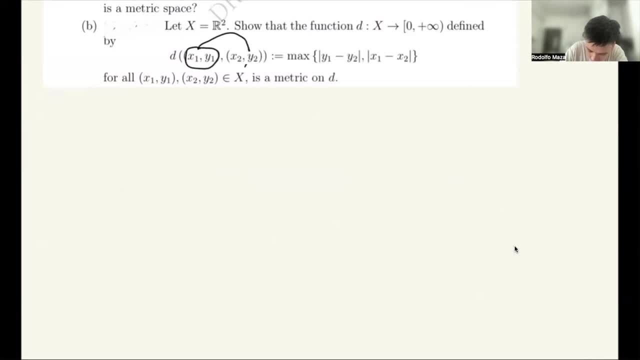 We can swap this, So kunyari, ito siya dyan and then this one is dyan, So diba, magsaswap lang yung location nila: Y2, Y1,, ito X2,. 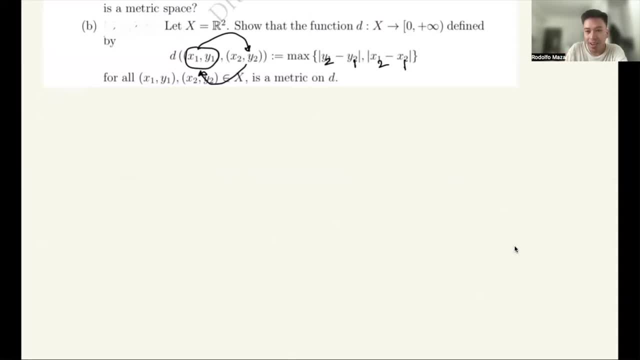 Y1, and it's still the same. Kasi, ano siya naka-absolute value naman, So pwede mo siyang iswap. Although it's negative, it's still the same having result. And for 3,. 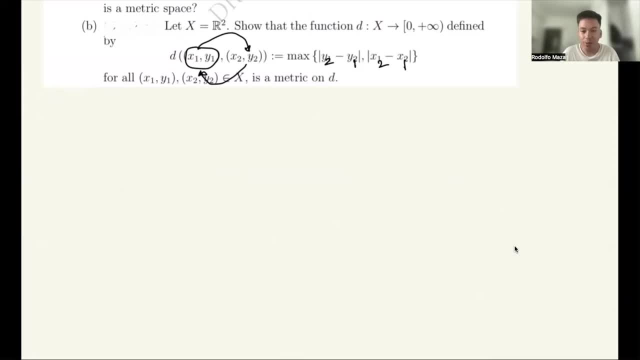 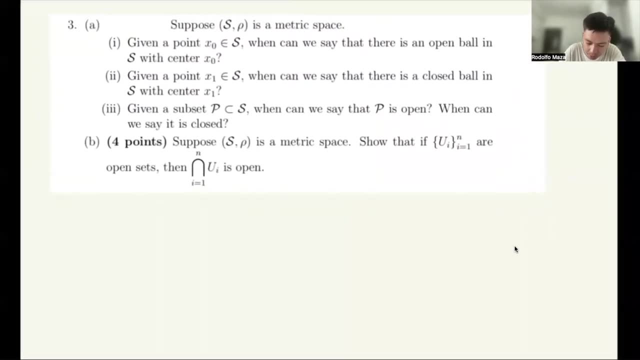 pwede mo siyang ia-add, and that's already a metric space. So that's it. It's pretty obvious, Number 3.. To pose S: P is a metric space, S row. So given a point, X, sub 0 and S. 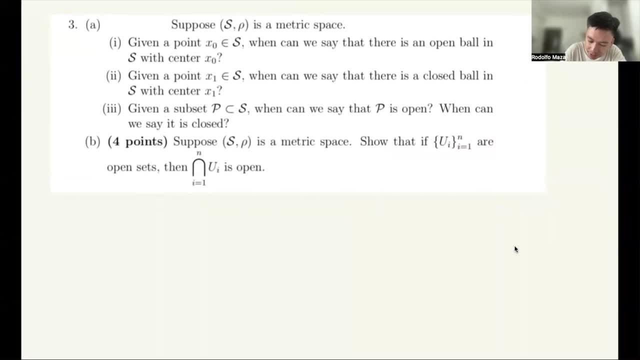 when can we say that there is an open ball in S with a center X sub 0?? So letter I. So we say there is an open ball in S with center at ano, yung center niya X sub 1,. 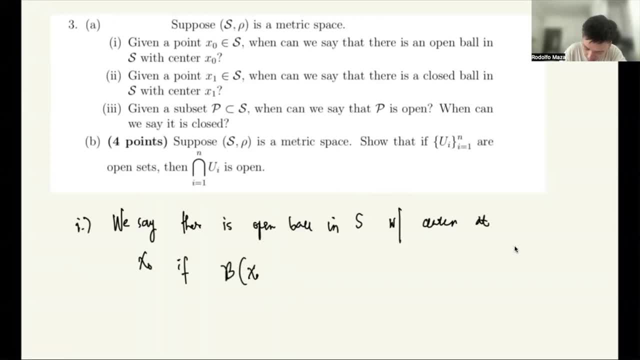 ah, X sub 0, if B of X sub 0 delta is equal to X in S, such that X row of X, X sub 0 is less than delta for any delta Greater than 0.. Okay, For number 2 naman. 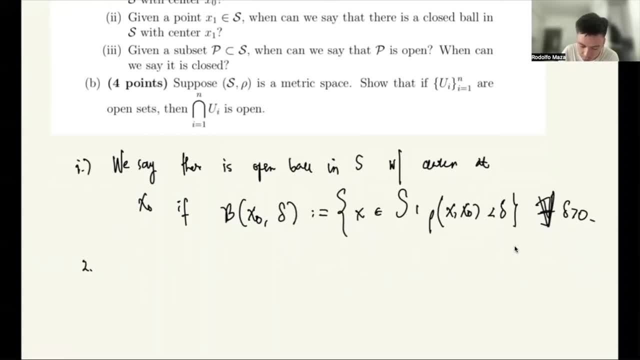 or double. I given X sub 1, when can we say there is a closed ball? So mangyayari? we say na may closed ball siya with center at X sub 1, if B of X sub 1 delta. 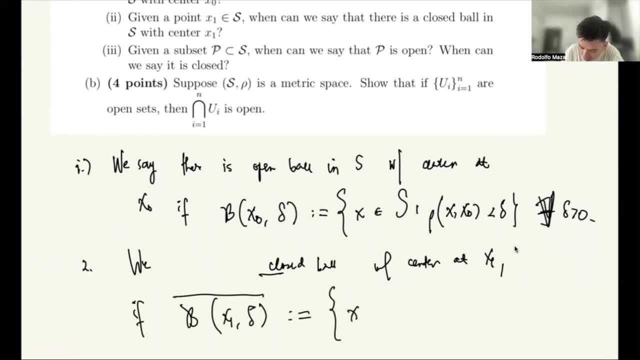 yan. this contains the set of X in S, such that row of X X and center of X sub 0, 1 is less than or equal to delta. So ito lang yung pinakaiba ng open at close. 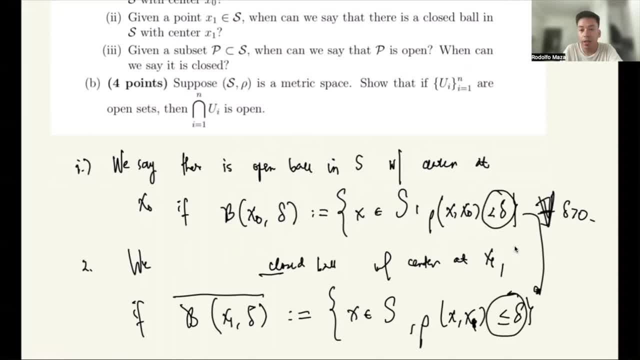 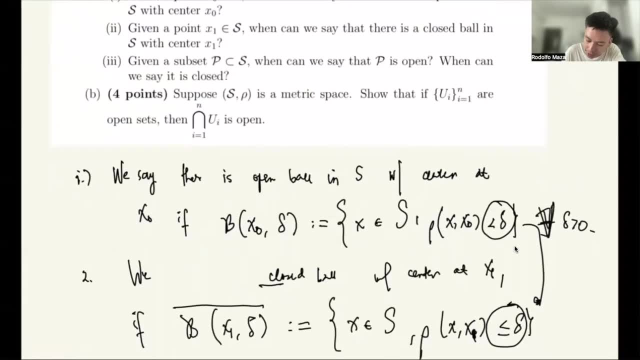 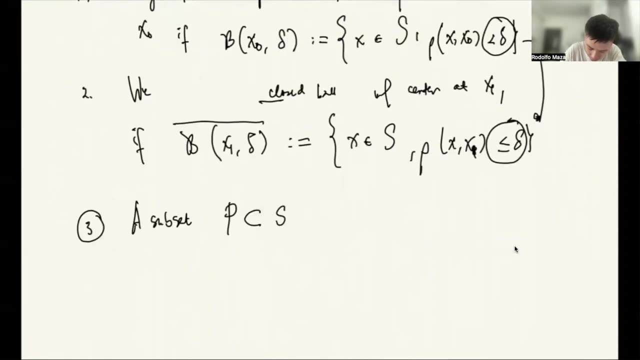 Yung open, kasi strict siya. Dito naman is less than or equal. Okay for number 3, when can we say that P is open and then P is closed? This is a subset of a metric space, A subset. P subset ni S is open. 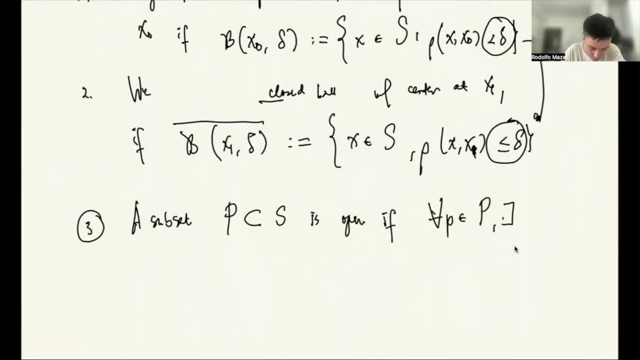 if for every P in P there exists a radius, let's say R, greater than 0. You know, your R is dependent on P, such that yung open ball PR is a subset of P. So ibig sab pihin. 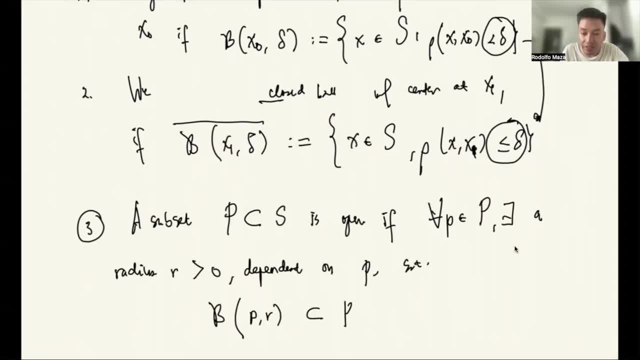 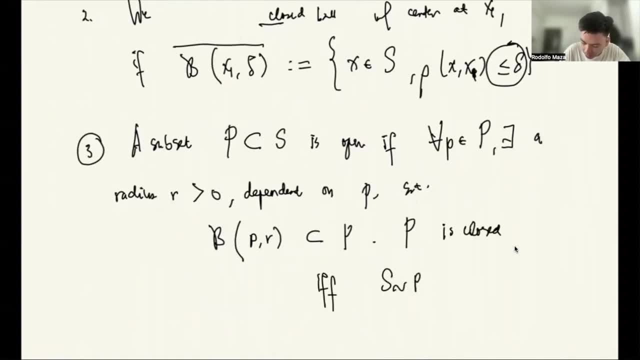 it's the other way of saying a subset, P, is open if it contains an open ball. So P is closed if, and only if, S minus P or the complement of P is open. That's it So if you have any questions or clarifications. 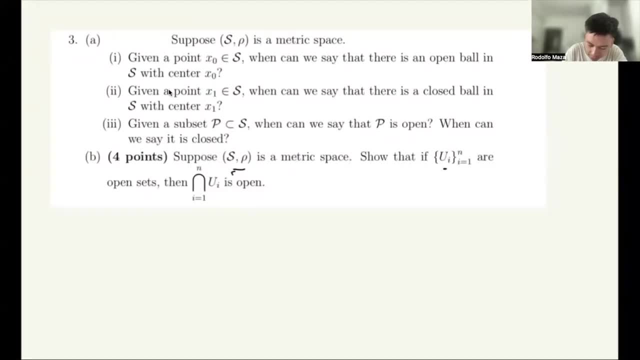 please let me know. Okay, number 4.. So suppose S, this one is a metric space. show that if the union of all U, I, I, from 1 to N, are open sets, are collections of open sets, is a collection of open sets. 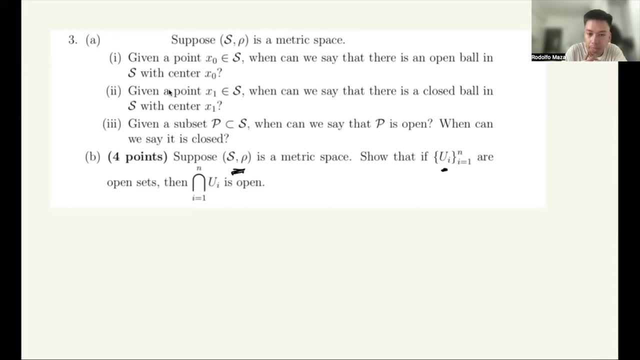 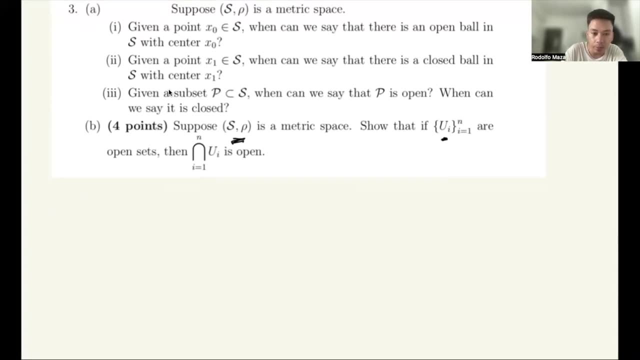 then the intersection of U, I is open. So paano natin yan isosolve Diba para magiging open sets, ibig sabihin it contains an open ball. So fix muna tayo, fix P. 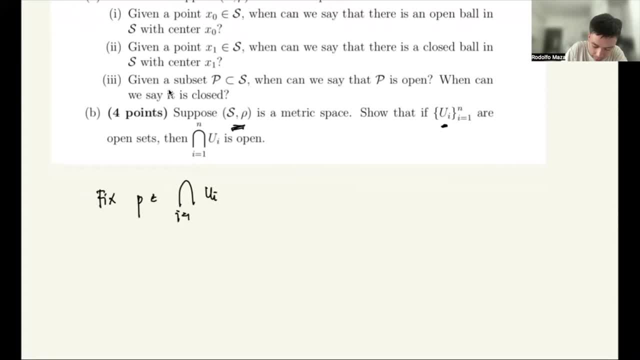 element of the intersection of U I, I from 1 to N, then ano to for all I from 1 to up to N. yung P mo is in U I Kasi. alam natin kasi na. 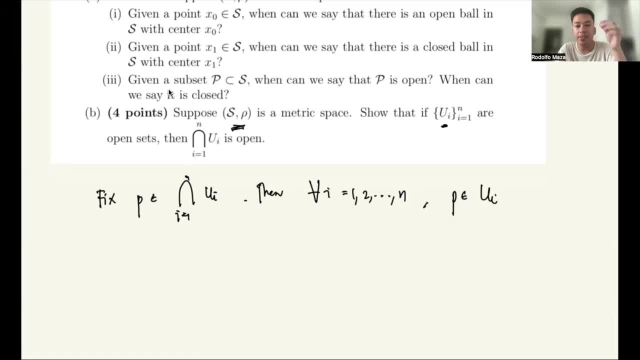 diba, element sya ng intersection, so ibig sabihin element sya sa bawat elements na yun. Anong mangyayari yan? Since yung U I mo kasi is open for all I. 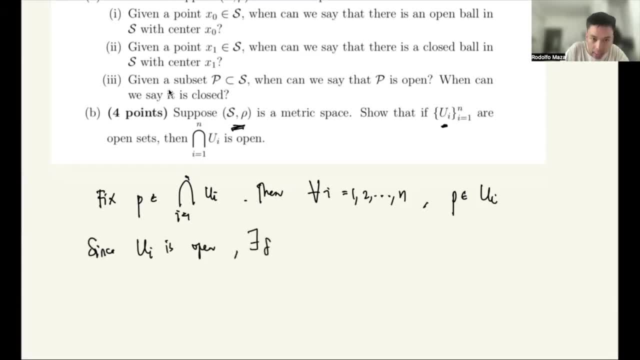 there exists a delta I, such that yung B of P delta I is in the U. I Kasi alam natin this is open, ibig sabihin ang pagiging open nito. 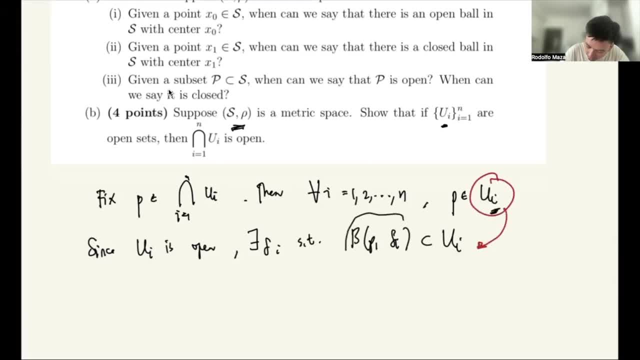 nagkocontain ng open ball which is nakakreate tayo ng open ball there sa P. Okay, So let, anong gagawin natin? Let delta be the minimum of all the I, such that your I is from 1 up to N diba. 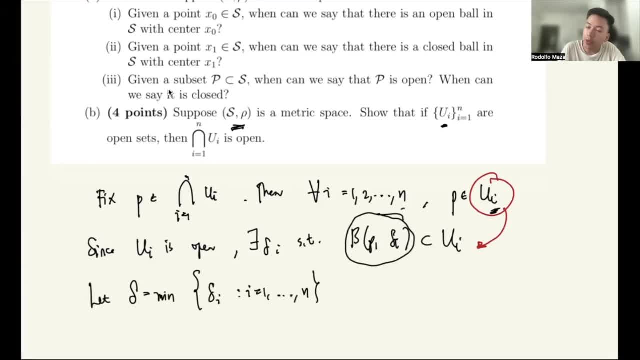 N tayo Okay, good N So kailangan natin kunin yung minimum, kasi kukuha lang naman tayo ng pinakamaliit doon, eh. So anong implication Then? your delta is greater than 0,. 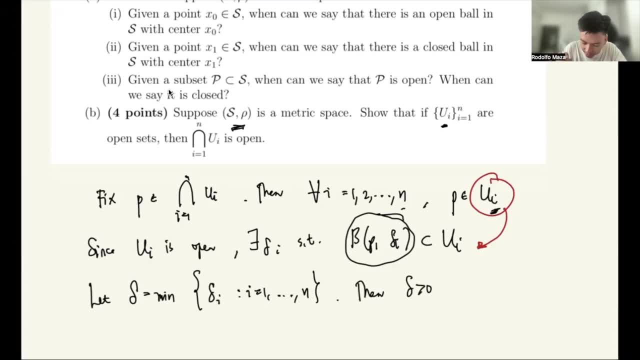 kasi sya yung minimum, pero lahat ng elements ng delta, lahat ng delta I mo should always greater than 0, para makakreate ka ng open ball. Okay, Then gagawa tayo ng open ball. 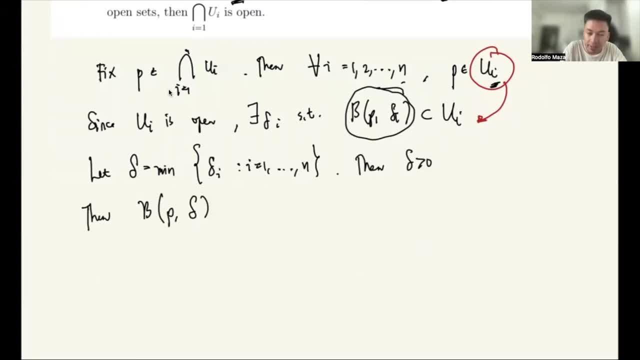 P of delta, Kasi si delta is a minimum of all the delta I's ibig sabihin this is a subset of B of P, delta I for each I from 1 to N diba Dahil. eto is a subset of these. 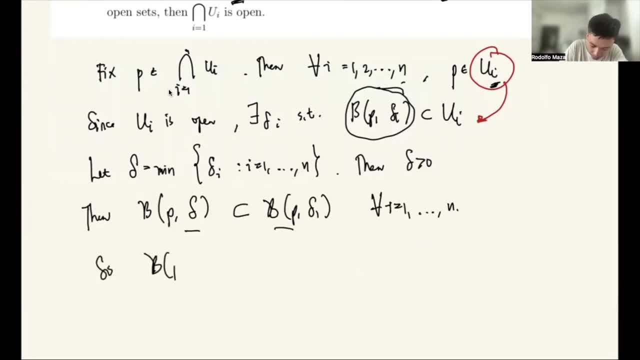 so B of P delta is in the intersection of UII from 1 to N, So dahil nagkunti na sya ng open ball na yan. so therefore mag-conclude na tayo that this one is open. 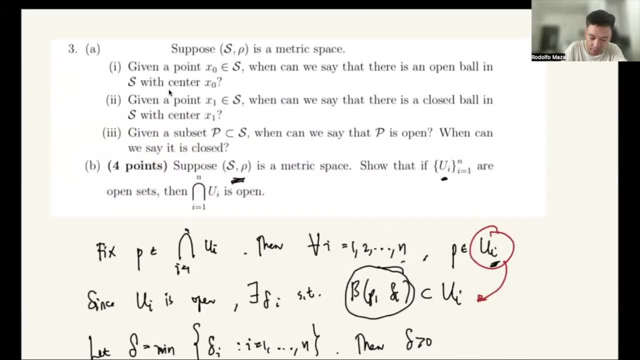 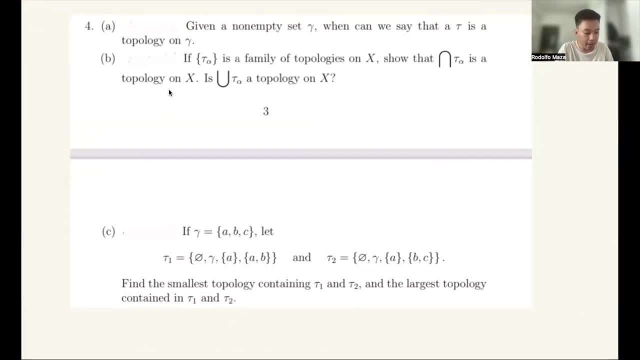 Yun lang. That's it. So that answers this one. Okay, number 4.. Given a non-empty set, gamma, when can we say that a tau is a topology on gamma? Okay, so it is a definition of topology. So paano natin. 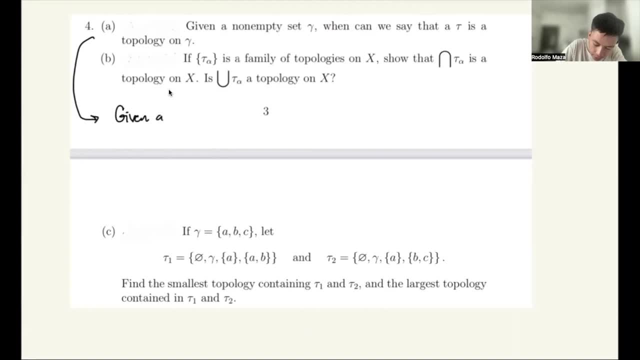 Given a non-empty set. tau, gamma- sorry, a tau is a topology on gamma. if, of course, tau is indeed a collection of subsets of gamma, of course this should be a collection first requirement, such that number 1,. 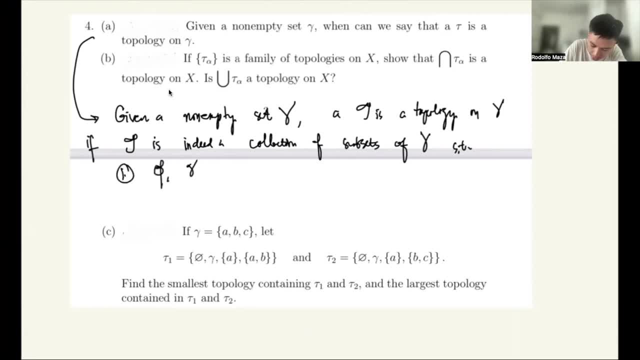 the empty and the gamma is in tau. Number 2, if the script U is a subset of tau, then the intersection of all U, your U, is an element of the script. U is in tau. So it's actually, I'm sorry. 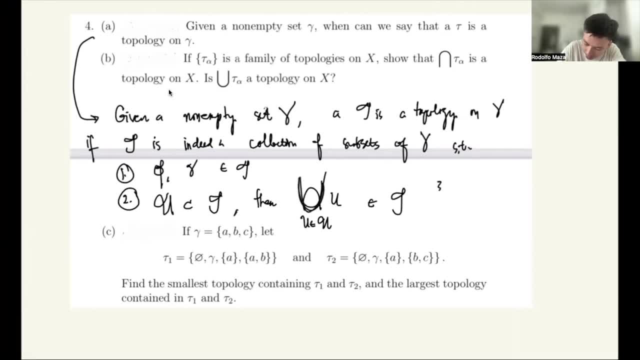 it should be union, It should be a countable union. And number 3,: if U1 until UK are in tau, then the finite intersection of all U i from 1 to N is in tau. So first the empty and the gamma are in tau. 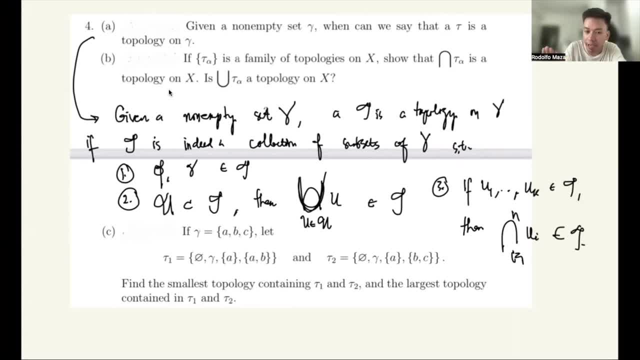 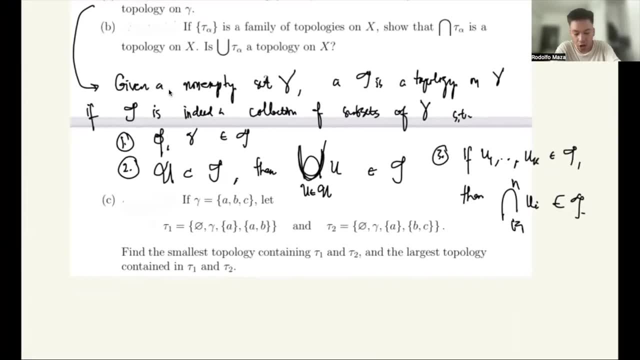 Second, the countable union and then the finite intersection. Okay for letter B. if tau sub alpha is a family of topologies on X, show that the intersection of tau sub alpha is a topology on X and is the union topology on X. 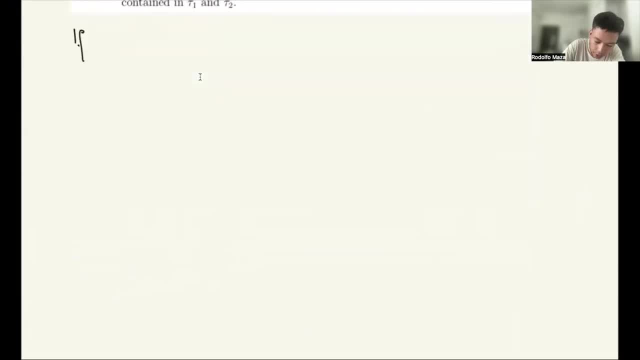 Okay, How do we prove that? Okay, So, if this one is equal to tau sub alpha, So what does this mean? Isn't tau sub alpha a topology? Because this one? because we know that tau sub alpha is a collection of topologies. 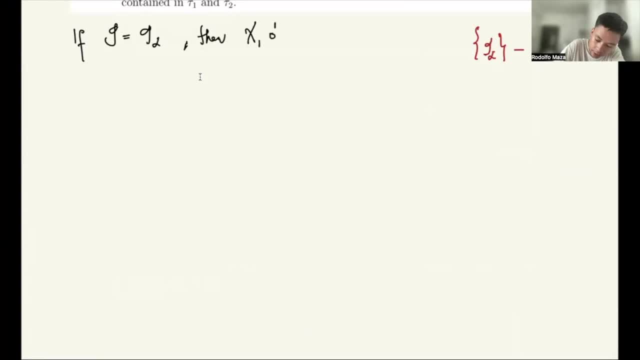 So that means X and the empty are elements of tau. Okay, Because it contains all the alpha. I mean it contains all the empty and the X in each alpha. Okay, now suppose this one is an index. 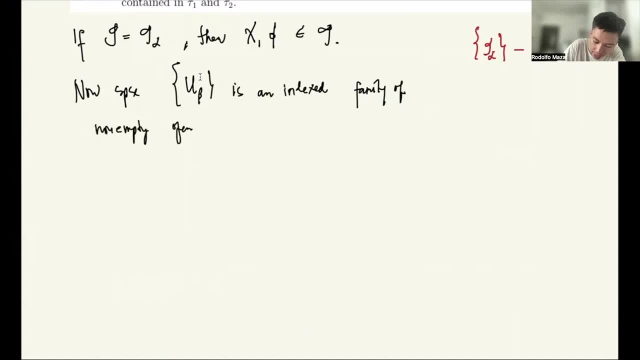 family of non-empty open sets in tau. Okay, So what happens then? So it means U of B is an element of tau sub alpha, And this is for each alpha Right. So your U is equal to the union of U sub B. 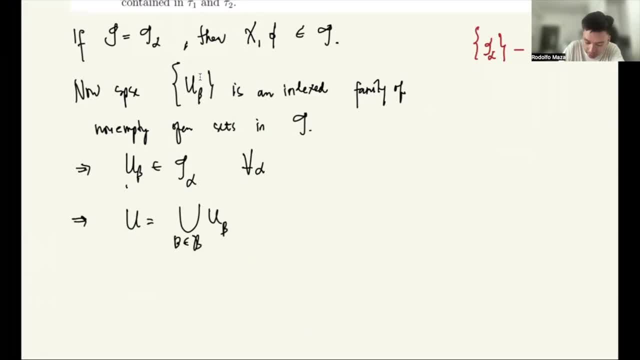 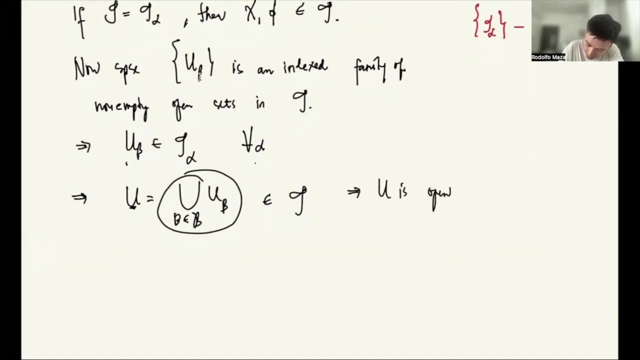 B in beta. It means because for all of them, this U here, which is the union of all of them, U sub beta, is an element of tau. So it means U is open, And so it's that way. 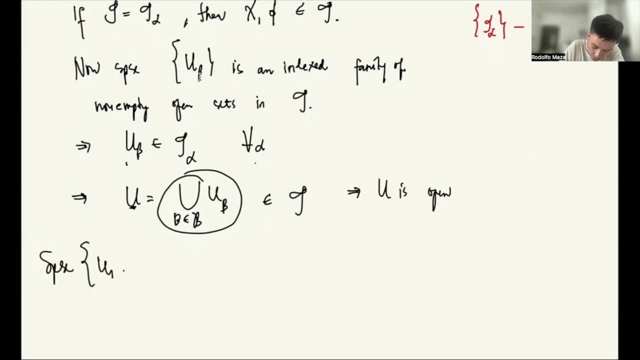 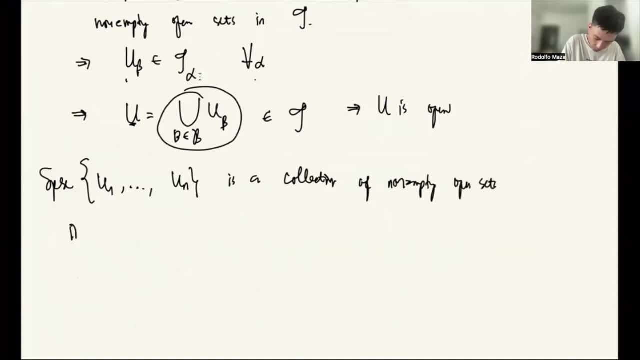 So, lastly, suppose U1 up until UN is a collection of non-empty open sets in tau. Okay, So, since U sub K is open in tau sub alpha and this is for all tau sub alpha, right. 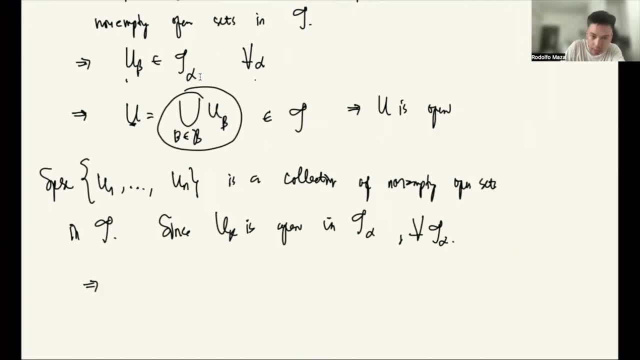 Okay, So it means your U. for example, let's put a label. let's say: U prime is equal to the intersection of U K K from 1 to N. So U K is open in tau sub alpha. 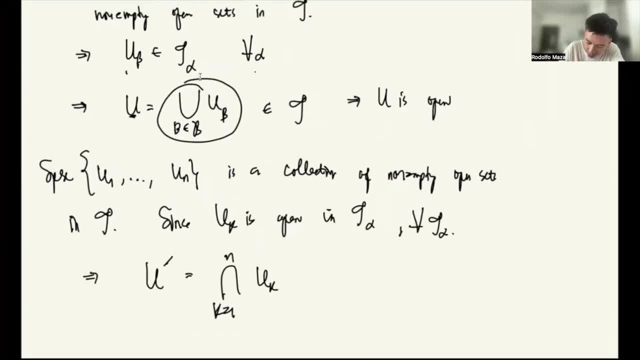 and that's for all alpha. So it means its intersection is open. so this is an element of tau sub alpha. So it implies that U sub K is an element of tau. Therefore, therefore, it's really a topology. That's it. 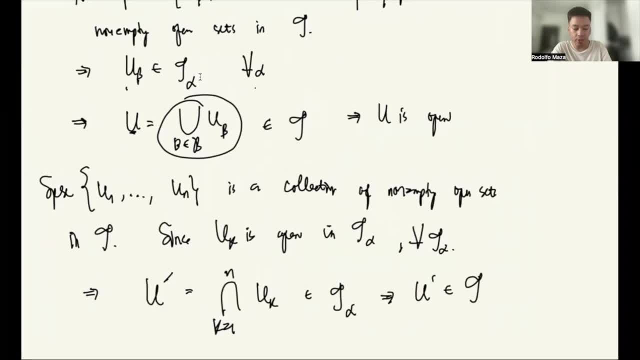 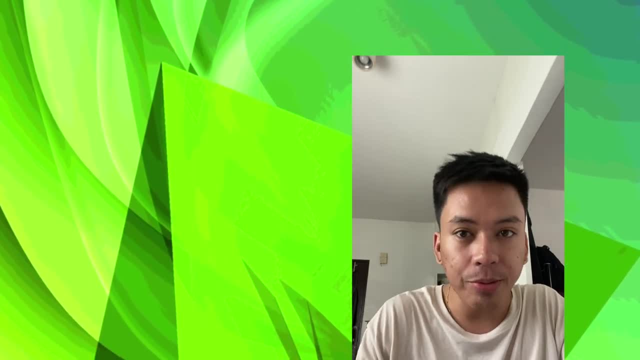 So, guys, if you have any questions or clarification, please let me know. Okay, that's all for today and thank you so much for watching. If you have any questions or clarification, please let me know so that we can talk on that. 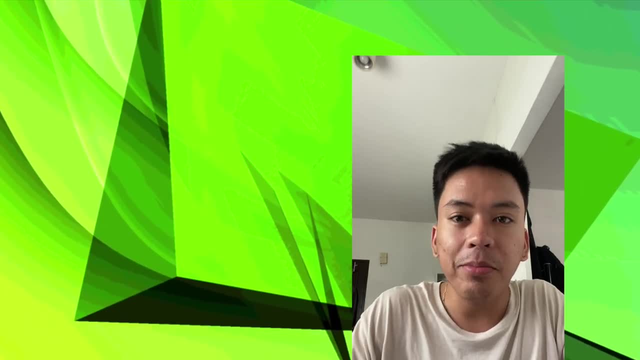 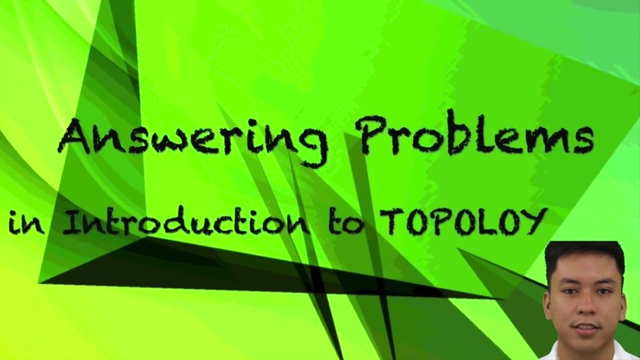 And if you are new to my channel, please don't forget to subscribe so that you'll be updated on a lot of videos that I'll be uploading soon. Thank you, Have a great day. Subtitles by the Amaraorg community.